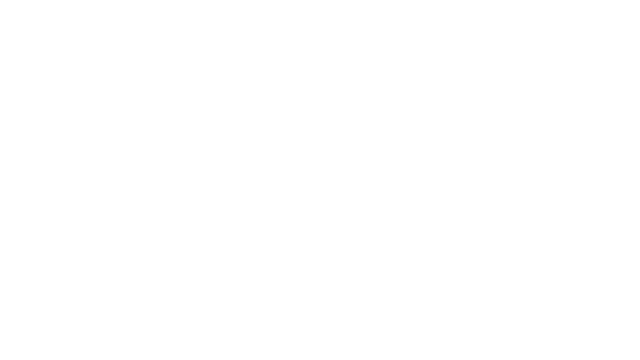 The d-h parameter table is a table that has one fewer rows than we have frames, because we have one row for each pair of frames. The table has four columns, one for each parameter. These four parameters include everything we need to express both the displacement and the rotation between two frames. 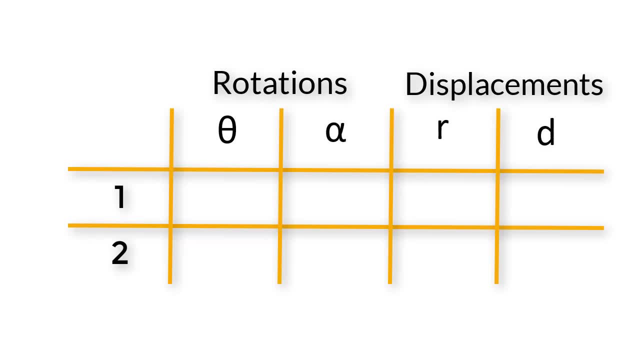 So if we know these parameters for each pair of frames, then we can get the homogeneous transformation matrix directly. Here is how it works. Two of the parameters record rotations and two parameters record displacements. I am going to define each one at a time and give an example for each to help you understand what the parameter means. 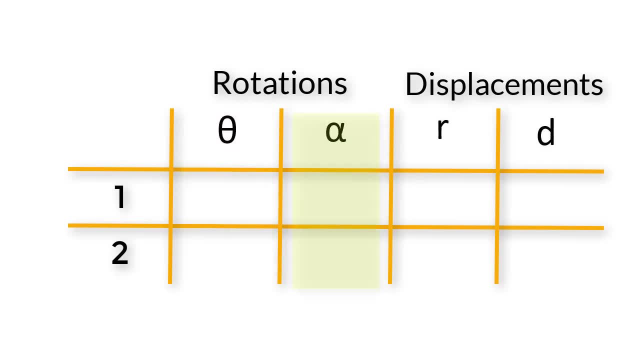 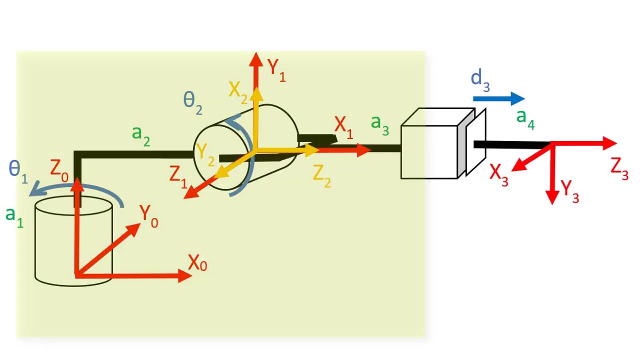 The four parameters are theta, alpha, r and d. Theta and alpha are rotation parameters and r and d are displacement parameters. Suppose we have two frames that are next to each other, like frame 0 and frame 1, or frame 1 and frame 2,. 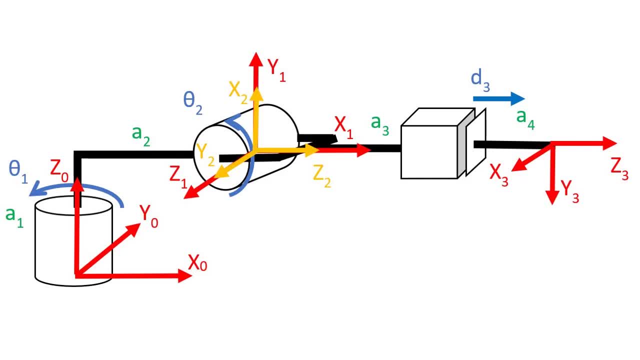 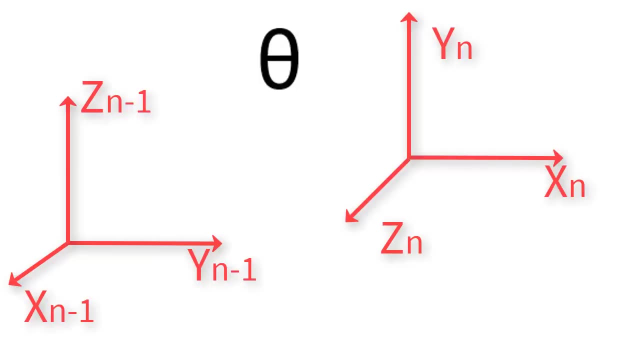 or something like that. Since this could apply to any two frames that are next to each other, I am going to call these two frames frame n and frame n-1.. Theta is the amount that we have to rotate frame n-1 around the axis in order to get axis to match the axis. 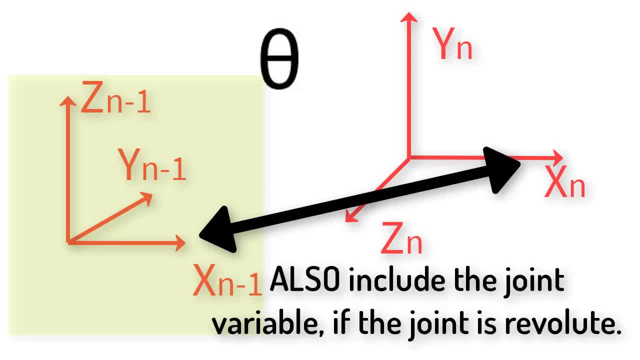 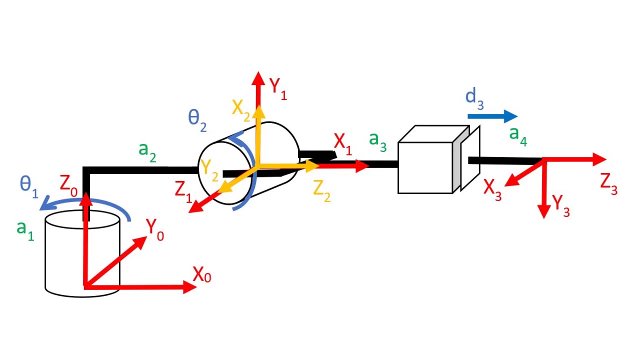 Also, we have to include in this parameter any rotation of the joint if the joint is a revolute joint, because this rotation is also a rotation around the axis. Let's try to understand this parameter better by looking at an example. Here is the kinematic diagram we drew in the last video. 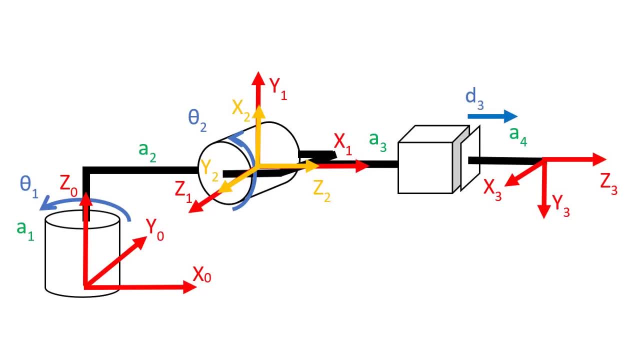 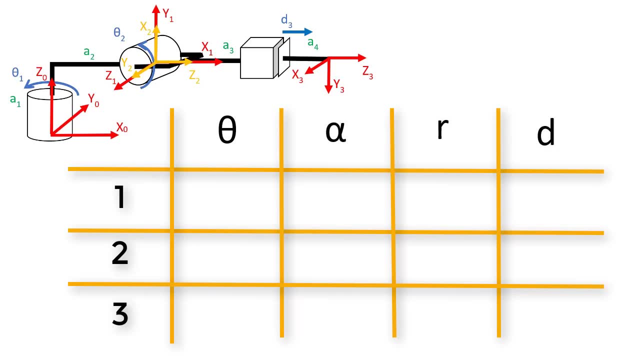 Here we have four frames, so we need to have three rows in our parameter table. We also have four columns, one for each parameter. The first two parameters are the rotational parameters. The first two parameters are the rotational parameters theta and alpha. 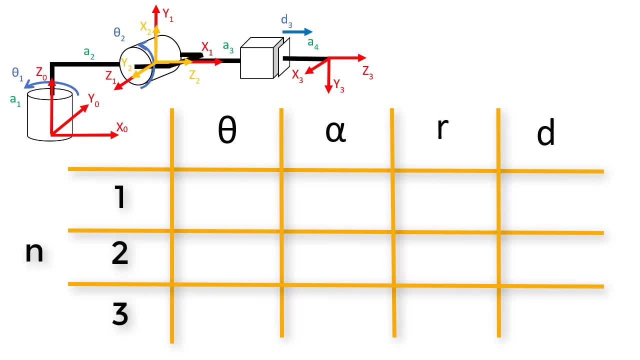 The rows are labeled for the value of n. so we have 1,, 2, and 3.. So we have 1,, 2, and 3.. Let's apply the definition of theta to the first row here. Let's apply the definition of theta to the first row here. 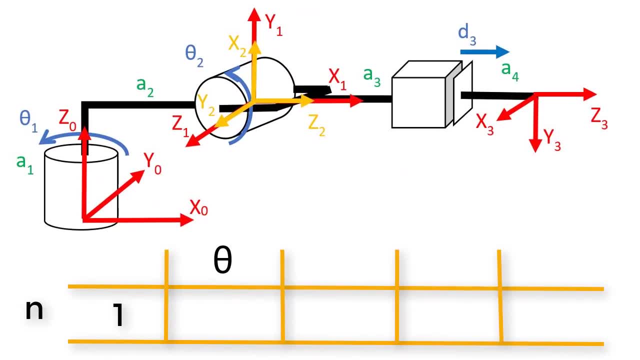 We'll substitute n equals 1, because this is row number 1.. Theta, then, is the amount that we have to rotate. theta, then, is the amount that we have to rotate frame 0 around the axis in order to get axis to match the axis. 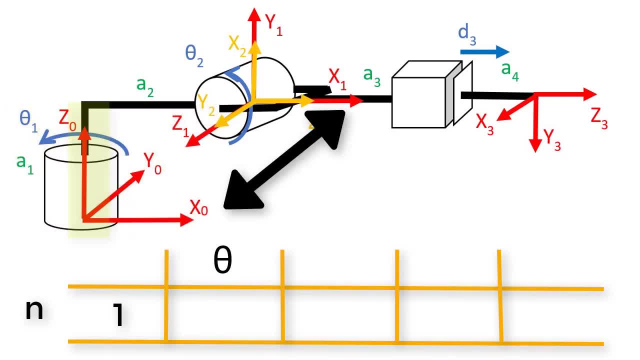 frame 0 around the axis in order to get axis to match the axis order to get axis x0 to match axis x1.. In our diagram, x0 is pointing to the right and x1 is also pointing to the right, So we don't have to rotate frame 0 at all in order to get axis x0 to match axis x1. 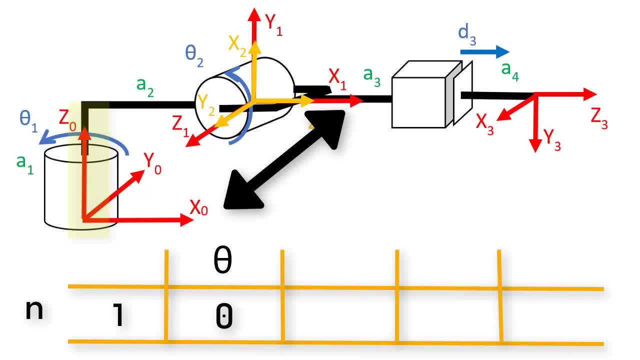 Let's write 0 here. but wait, there's one more thing for theta. We have to also include in this parameter any rotation of the joint, if the joint is a revolute joint, because this rotation is also a rotation around z0.. 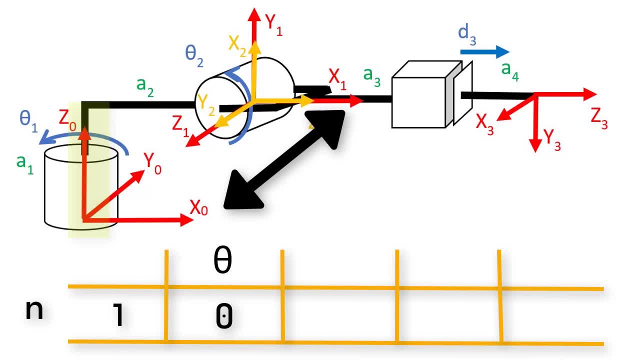 The rotation here is theta1, so we have to add that to this parameter. here The theta parameter for the first row is 0 plus theta1.. Let's do theta for the next row. Here n equals 2, because this is the second row of the table. 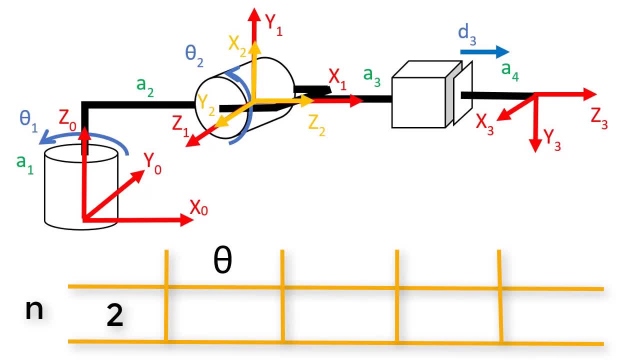 So theta is the amount that we have to rotate frame 1 around axis z1 in order to get axis x1 to match axis x2.. Here x1 is pointing to the right and x2 is pointing to the left, So theta is pointing up. 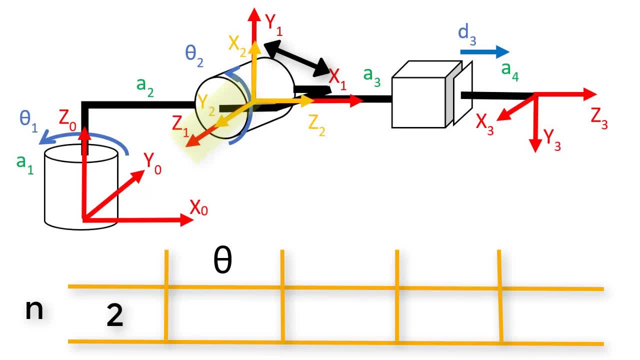 In order to get x1 to match x2, we will need to rotate frame 1 90 degrees. But should that be a positive 90 degrees or a negative 90 degrees? The axis we are rotating around is z1, and z1 is pointing out of the page towards us. 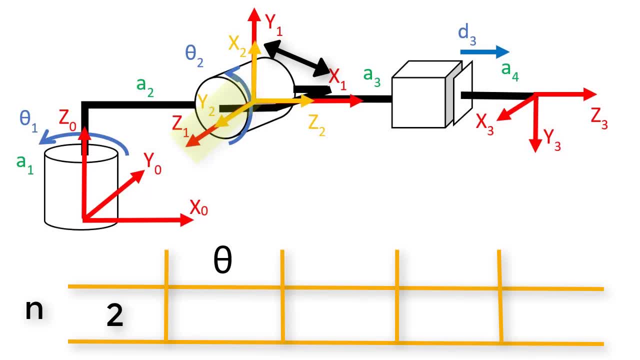 Using your right hand, point your thumb towards yourself and look at what direction your fingers curl. They curl around counterclockwise, which is the same direction that we have to rotate x1 in order to get it to match x2.. So the 90 degree rotation is positive. 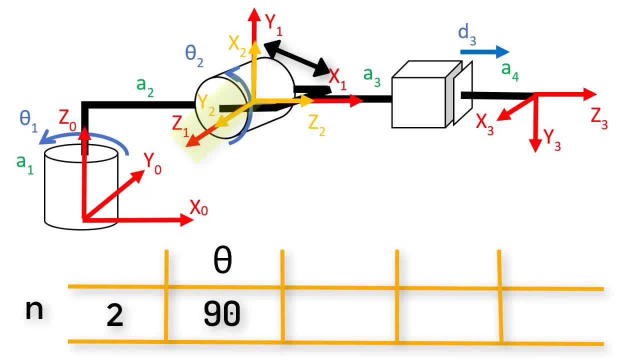 I am going to write 90 here, But wait, there is one more thing for theta. We also have to include in this parameter any rotation of the joint if the joint is a revolute joint, Because this rotation is also a rotation around z1.. 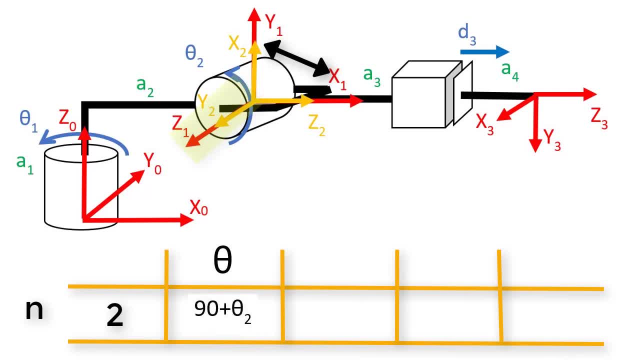 So I need to add on theta 2 here. Now let's do theta for the last row. Here n equals 3, because this is the third row of the table. So theta is the amount that we have to rotate frame 2 around the axis z2 in order to get. 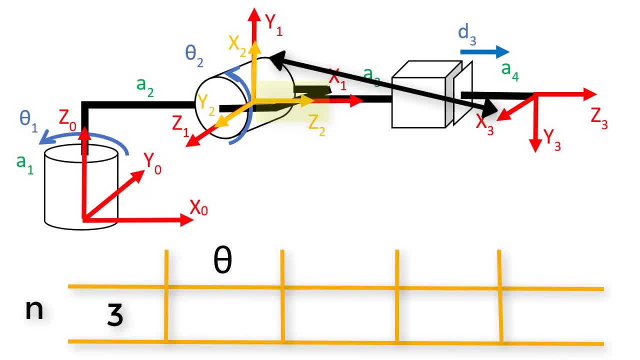 axis x2 to match axis x3.. Okay, Axis x2 is pointing up and axis x3 is pointing towards us, out of the page. So we need to rotate x2 90 degrees to get it to match. But should that be positive or negative? 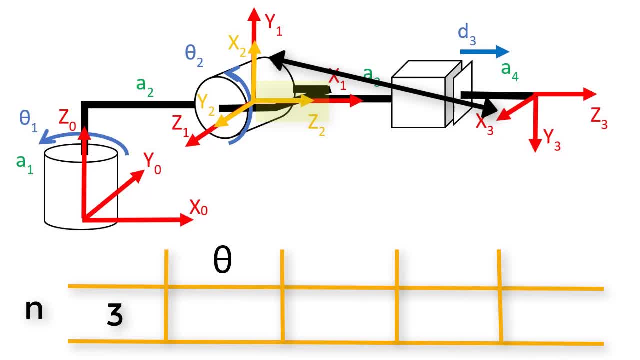 To find out. we put our right hand thumb in the direction of z2, to the right. The direction our fingers curl is the same direction that we want to rotate x2.. It's towards us. So the 90 is positive. I'm going to write 90 here. 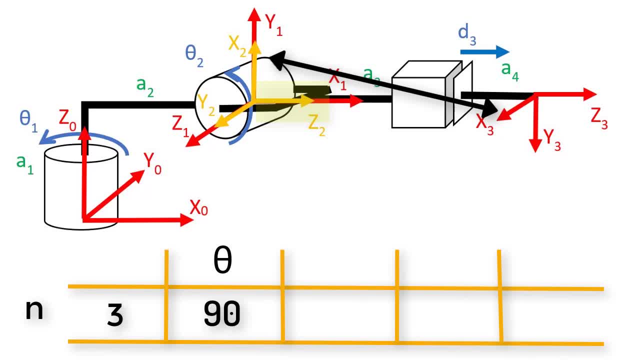 But wait, there's one more thing for theta. We also have to include in this parameter any rotation of the joint if the joint is a revolute joint. But this joint isn't a revolute joint, So the 90 that we wrote is all we have here. 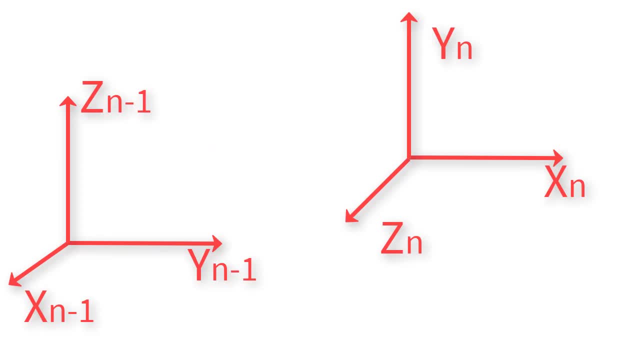 All right, Let's move on to the second parameter, Which is also a rotational parameter. It's called alpha. Alpha is the amount that we have to rotate frame n minus 1 around axis xn to get axis zn minus 1 to match zn. 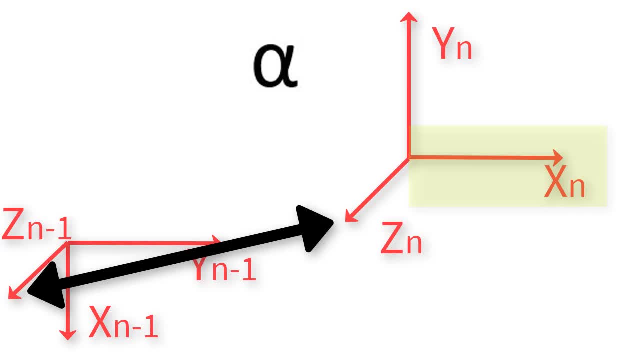 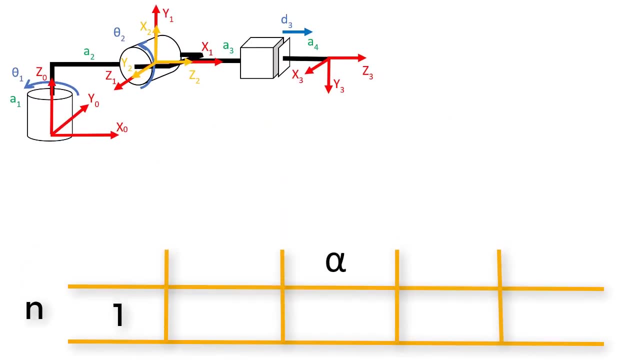 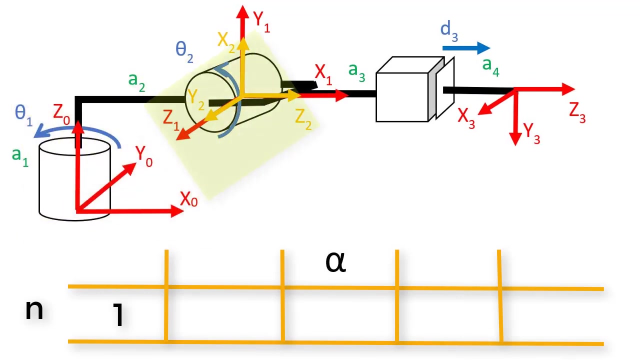 Let's do an example with the same kinematic diagram. For the first row we substitute n equals 1. So alpha 1. It's the amount that we have to rotate frame 0 around the axis x1 in order to get z0 to. 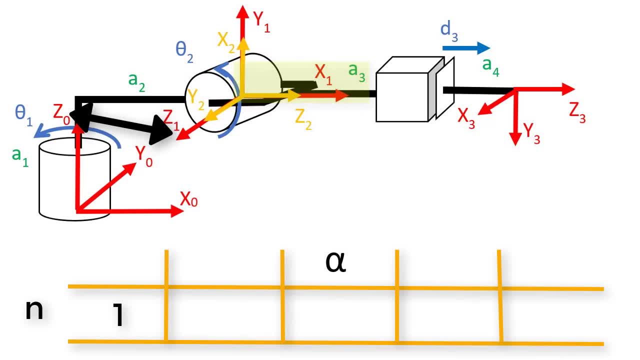 match z1.. This is a little bit tricky because you have to remember that the axis we're rotating around is x1, not x0. But the frame that we're rotating is frame 0. Not frame 1.. So, for example, z0 is pointing up and z1 is pointing out of the page towards us. 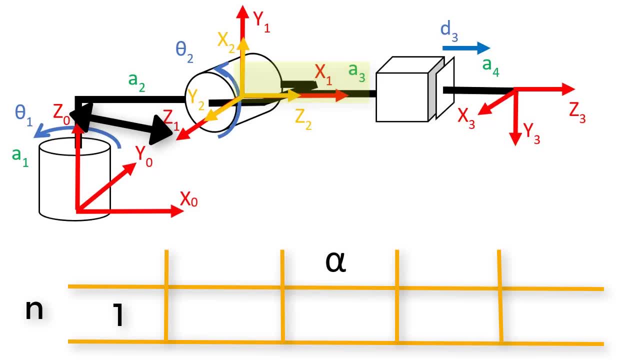 So we have to rotate frame 0 90 degrees to get z0 to match z1. But should this be a positive 90 or a negative 90?? To find out, we put our thumb in the direction of x1 and rotate it 90 degrees to get z0 to. 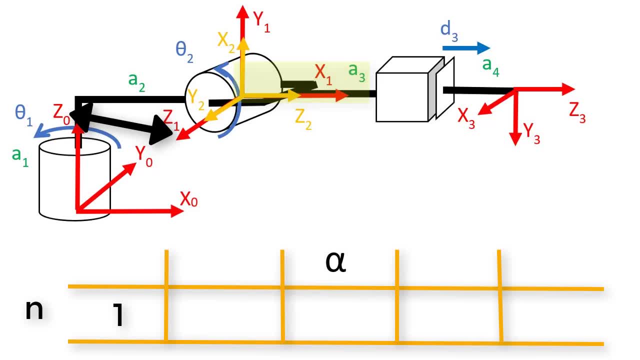 match z1. But should this be a positive 90 or a negative 90?? To find out, we put our thumb in the direction of x1 and rotate it 90 degrees to get z0 to match z1. But should this be a positive 90 or a negative 90?? 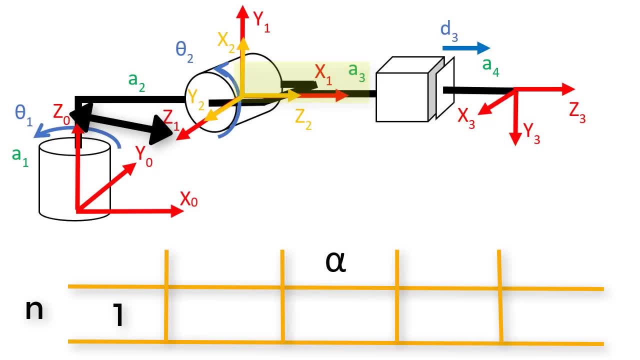 To find out, we put our thumb in the direction of x1 and rotate it 90 degrees to get z0 to match z1.. For this example, our thumb is pointing in the direction of x1.. To familiarize you all with the margin of the front, if the angle of our fingers were: 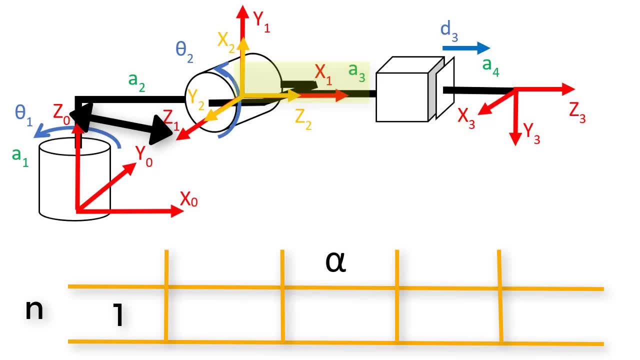 20 degrees to the side. For this example, our thumb is pointing in the direction of x1, so we justänático, singing feet right from the bottom makes us use our right hand and we look at the direction, our fingers curl, But we fürct over the line 90 degrees. 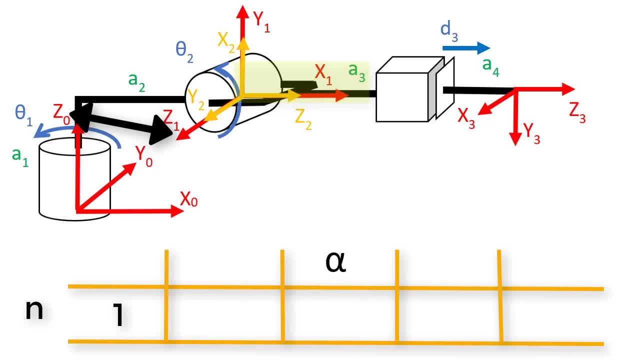 And now that we have our mask on, we have two lines in front again. The left bottom has its right and the left one has its left in this place in the table. Next, let's look at alpha for the second row. Since this is the second row, I'll substitute: n equals 2.. 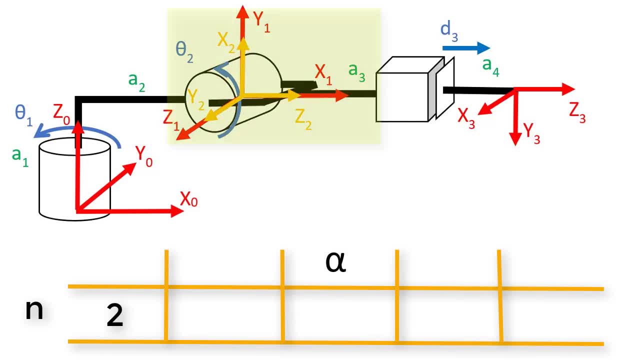 Alpha. here is the amount that we have to rotate frame 1 around the axis x2 in order to get axis z1 to match axis z2.. z1 is coming out of the page towards us and z2 is pointing to the right. 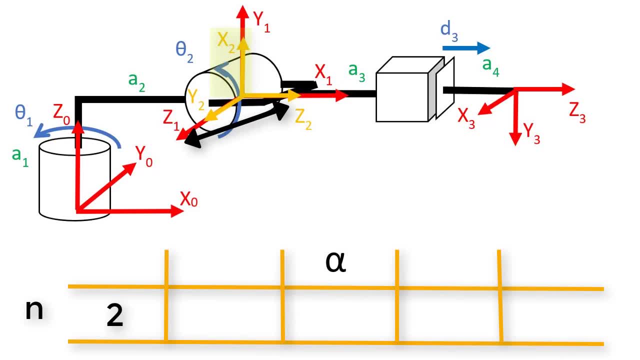 So we need to rotate frame 1 90 degrees in order to get z1 to match z2.. So should this be a positive or a negative 90?? We take our right hand and we put our thumb in the direction of x2, pointing up. 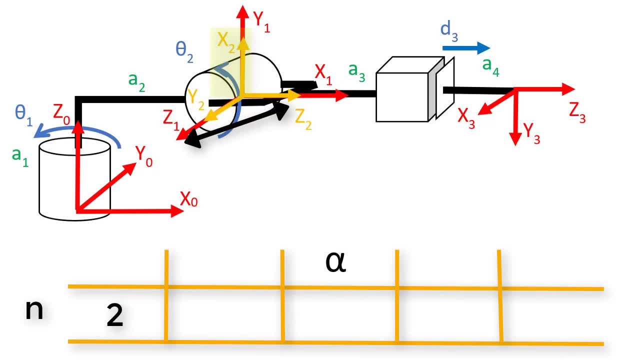 And we look at the direction that our fingers curl. Our fingers curl around. Our fingers curl around to the right. That is the direction that we need to move z1 in order to get it to match z2.. So the 90 degrees here is positive. 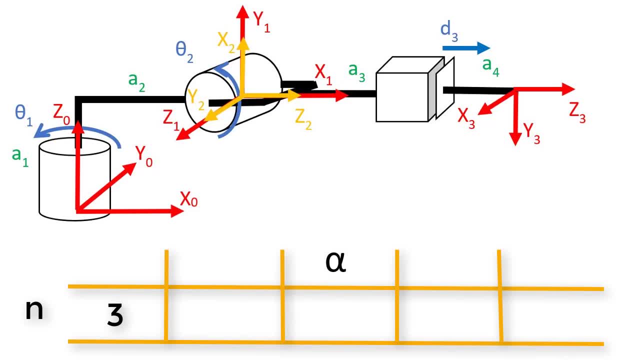 Now let's look at alpha for the third row. For the third row, I'll substitute: n equals 3.. Alpha is now the amount that we have to rotate frame 2 around the axis x3 in order to get z2 to match z3.. 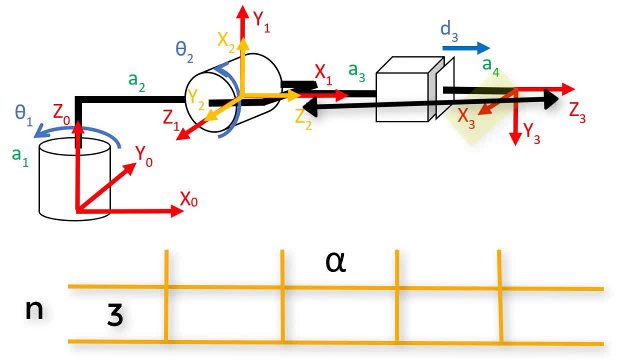 z2 is pointing to the right and z3 is also pointing to the right, So we don't have to rotate frame 2 at all in order to get these two axes to match. So I'll put 0 in here for alpha in the third row. 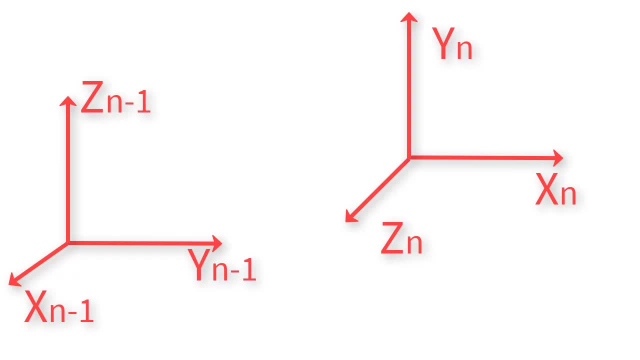 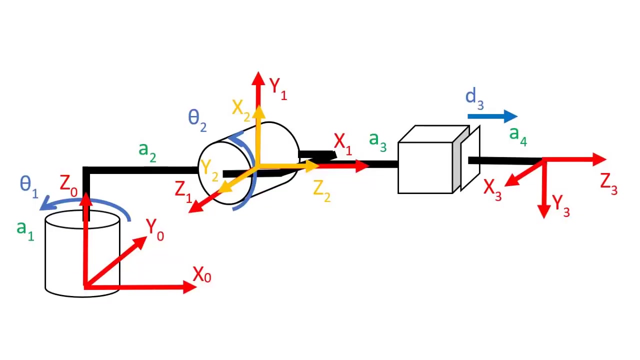 Let's move on to our first displacement parameter, r. Here's how r is defined: r is the amount of displacement from the center of frame n minus 1 to the center of frame n, measured only in the xn direction. Let's look at some examples. 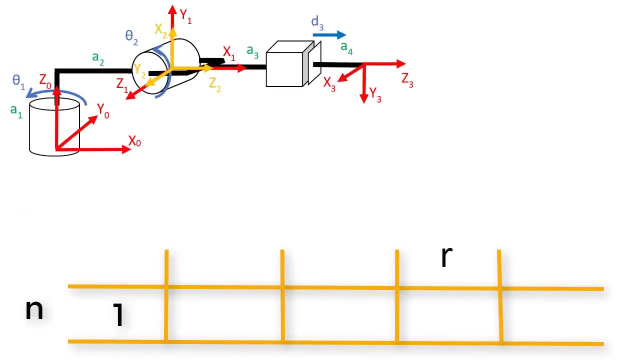 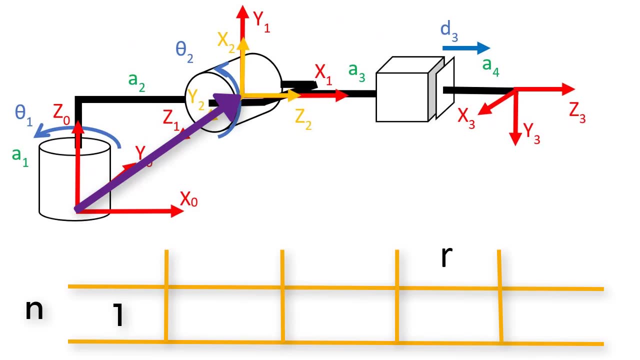 The displacement from the center of frame 0 to the center of frame 1. is this vector shown here? I want to write the component of this vector that is only in the x1 direction, The component of this vector that is in the x1 direction, which is pointing to the right. 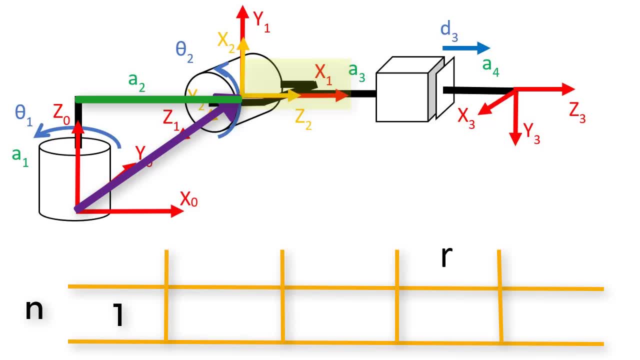 is the link length a2.. So I'll write a2 here in the table. Next we can move on to r for the next row. r for the next row is the displacement from the center of frame 1 to the center of frame 2, measured only in the x2 direction. 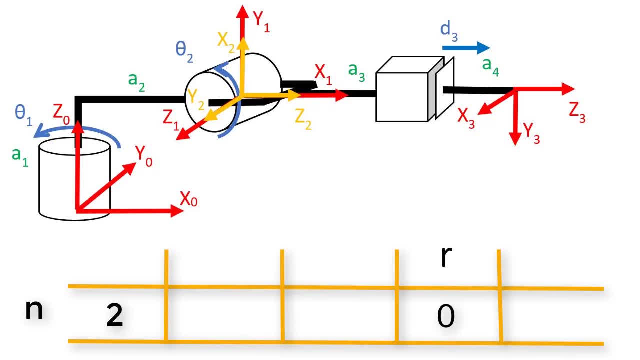 The displacement between these two frames is 0 because the center of the two frames are exactly on top of each other, So I write 0 in this place of the table. For the third row, r is the displacement from the center of frame 2 to the center of frame. 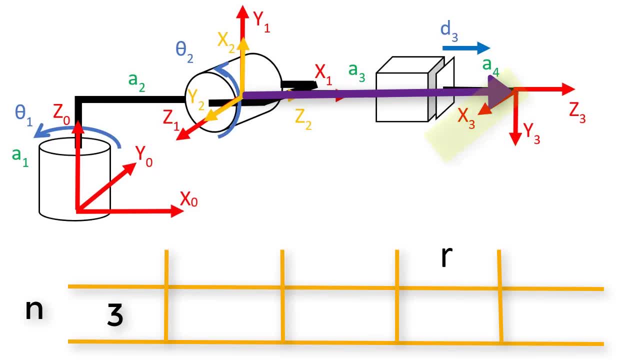 3, measured only in the x3 direction. The displacement from the center of frame 2 to the center of frame 3, measured only in the x3 direction. So I write 0 in this place of the table. The displacement between these two frames is 0, because the center of the two frames 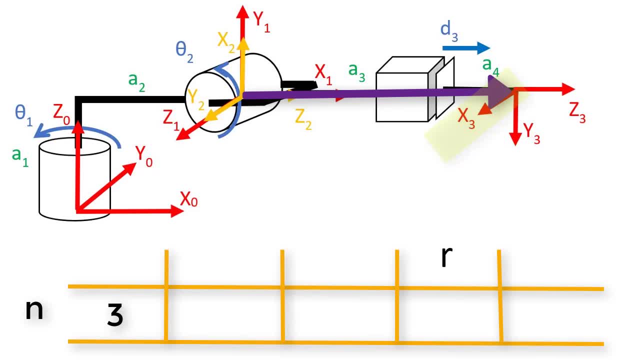 are exactly on top of each other. So I write 0 in the x3 direction. So I write 0 in this place of the table And we're finished with this parameter. Let's move on to the second displacement, parameter d. 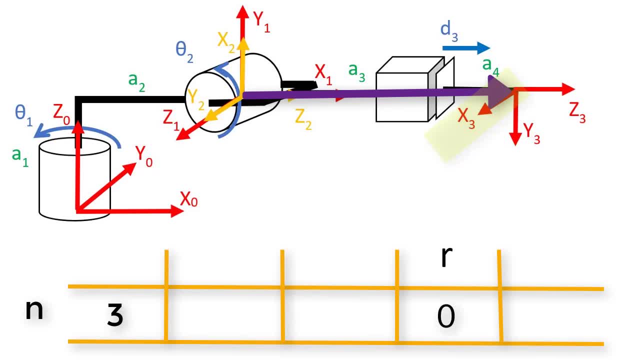 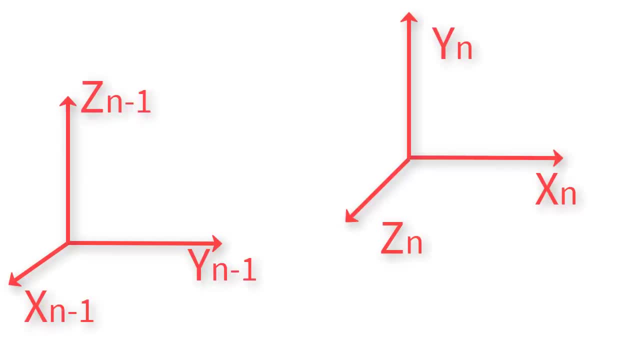 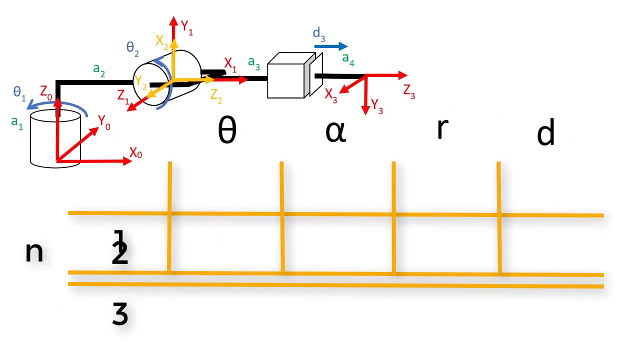 d is the amount of displacement from the center of frame n minus 1 to the center of frame n, measured only in the x3 direction, only in the z? n minus 1 direction. Let's look at some examples For row 1 I. 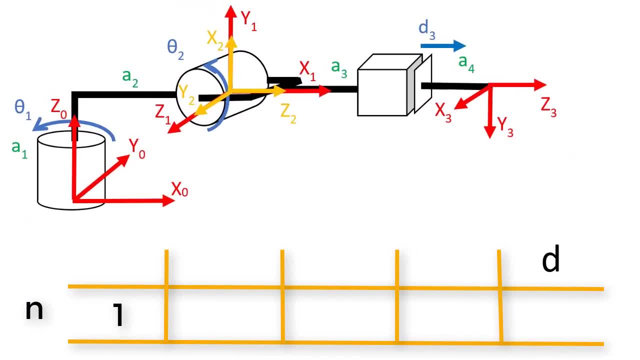 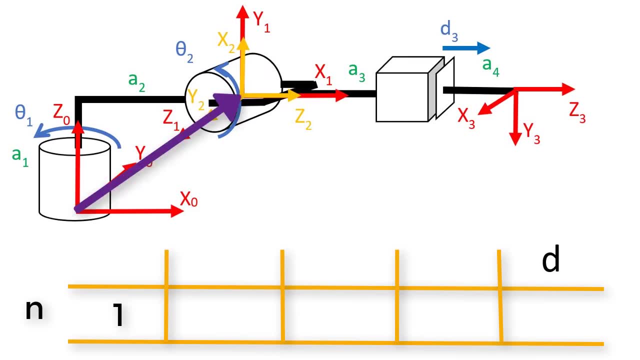 substitute in n equals 1.. So the D parameter here means the displacement from the center of frame 0 to the center of frame 1, measured only in the z 0 direction. The component of this vector in the z 0 direction is a 1.. So I'll 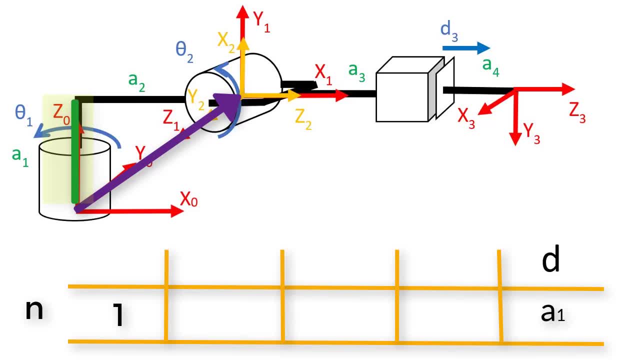 write a 1 in this part of the table. Next, let's do D for the second row. I substitute n equals 2 into the definition of the D parameter. D for row 2 is the displacement from the center of frame 1 to the center of frame 2. 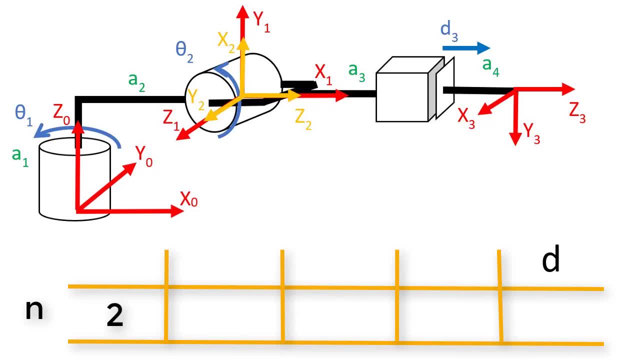 measured only in the z 1 direction. Now here, filling in this parameter is very easy, because the center of frame 2 is exactly in the same place as the center of frame 1. There is no displacement at all between the centers of these frames. 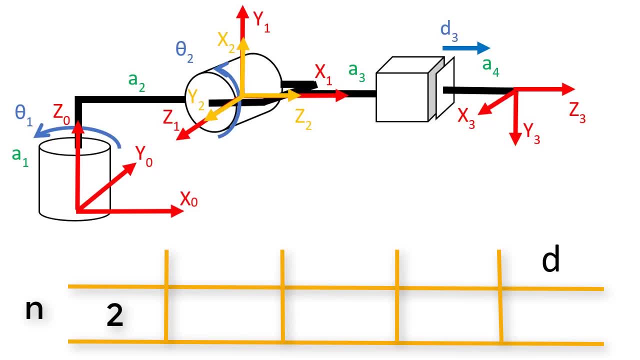 So, since there is no displacement at all, the z component is also 0 and I fill in 0 in this place at the table. Lastly, let's do the third row. I substitute in n equals 3.. D for the third row is the displacement from the center of frame 2 to the center of frame 3. 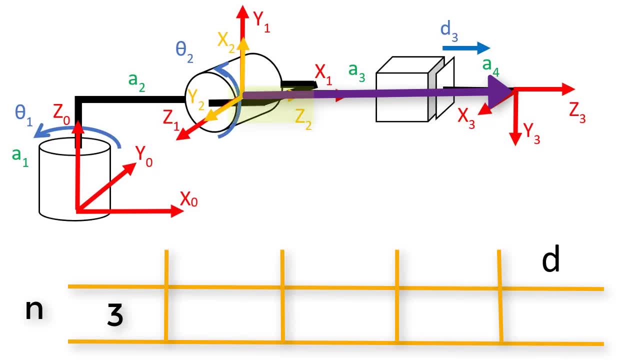 measured only in the z 2 direction. I have quite a few components of this vector to take into account. This displacement includes the lint in the z 2 direction, the link length A3, the link length A4, and also the joint variable D3. 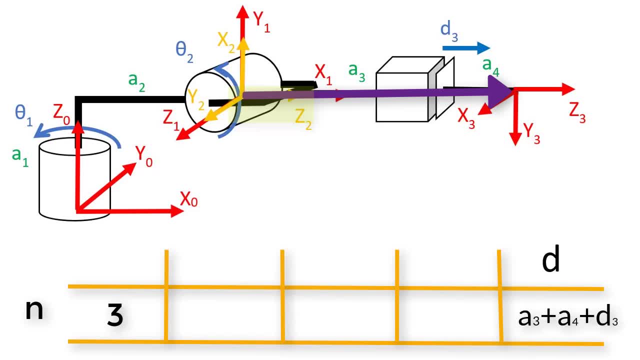 So in this part of the table I'm going to write in A3 plus A4 plus D3.. We've now finished filling out the table for this example. 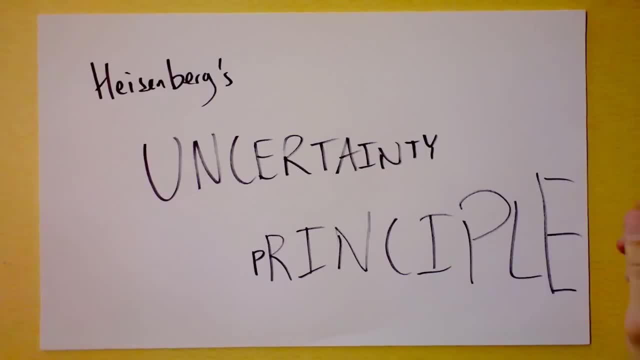 Heisenberg's Uncertainty Principle is one of the crowning achievements of quantum mechanics. We're kind of getting to a lot of the most important stuff right here, a lot of the coolest results. The Uncertainty Principle is something you may have heard of. actually It's that. 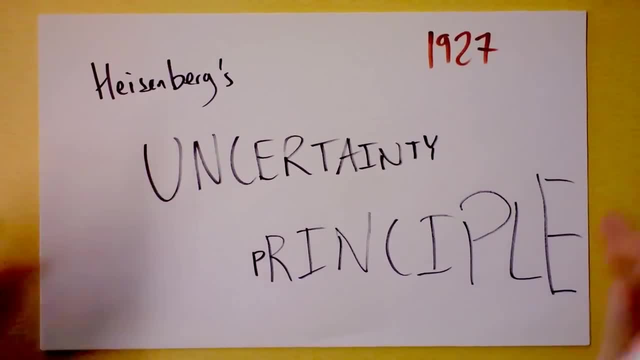 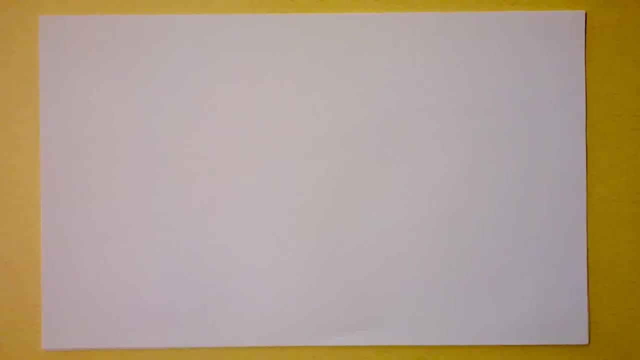 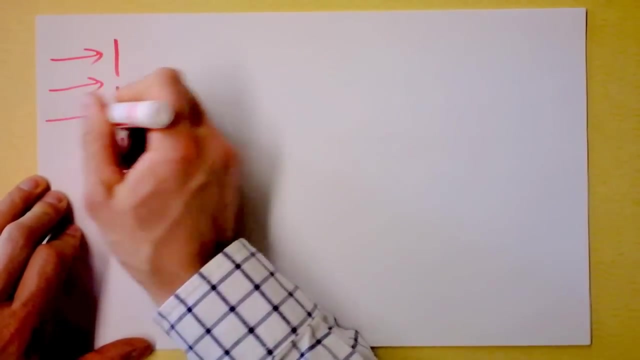 big of a thing. So 1927, this 26-year-old German named Werner Heisenberg comes up with this really, really interesting treatment. Let's see how this works. We recall, of course, that if we have electrons and they hit a double-slit apparatus like this—here I'm 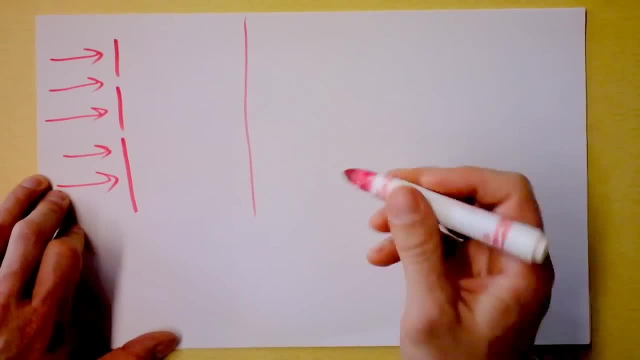 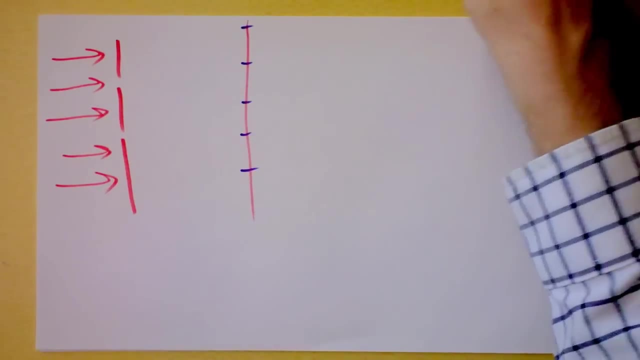 going to send in my electrons—then I'm going to get a fringe pattern over here. Let me try to draw it a little bit carefully. We've got some bright fringes and some dark fringes, and on this screen, let's say, there's a phosphor over here that's glowing every.